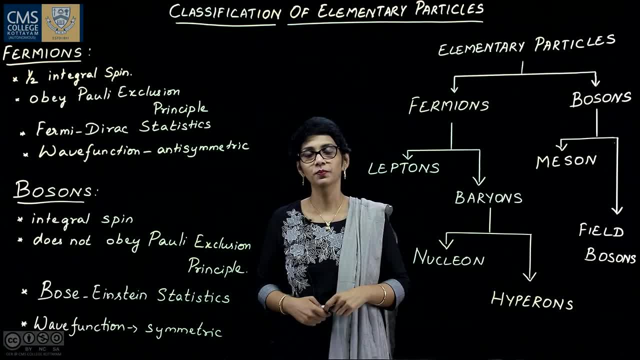 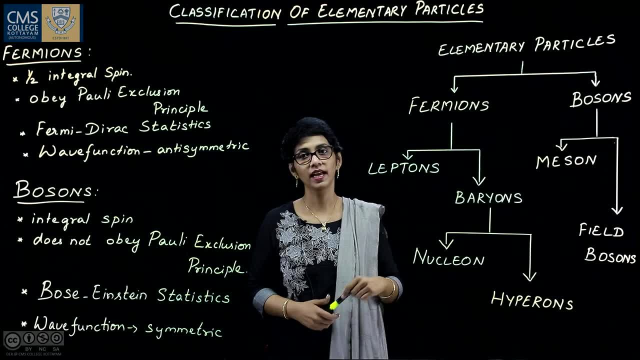 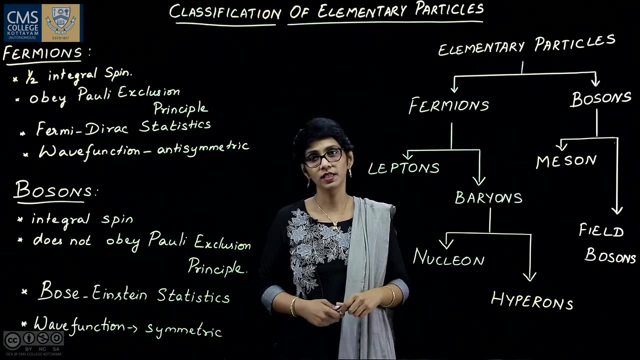 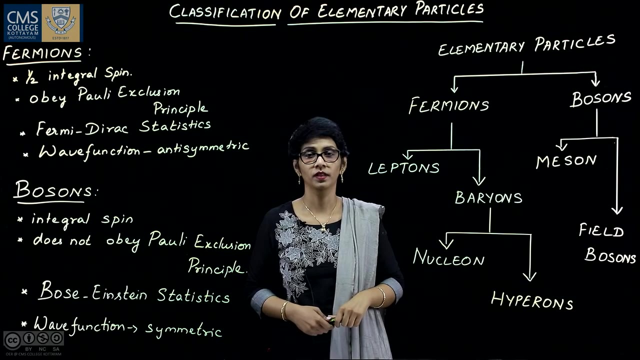 Hello everyone, Here in this video we are going to see the classification of elementary particles. Elementary particles can be grouped into two broad categories- fermions and bosons, based on the property called spin, which is connected by the kind of statistics the particles are governed by. Almost all elementary particles spin about the axis. 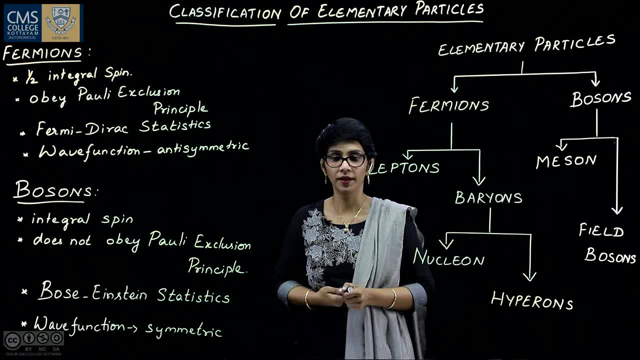 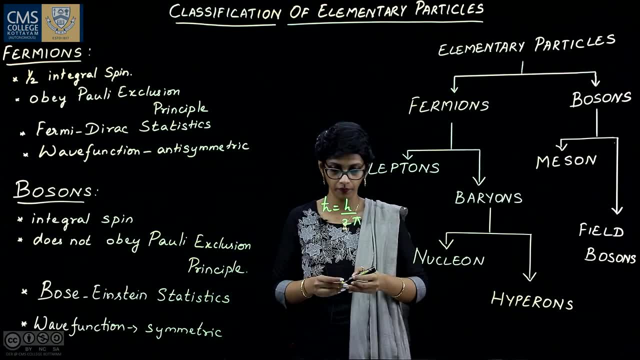 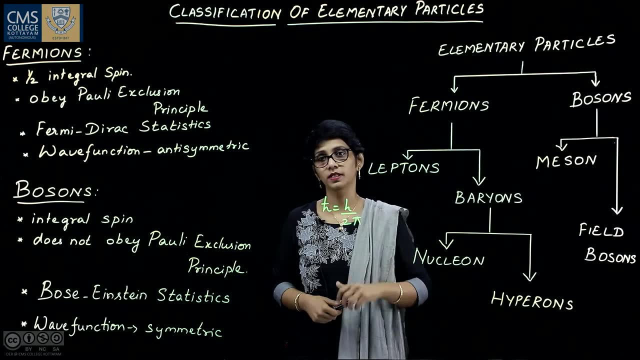 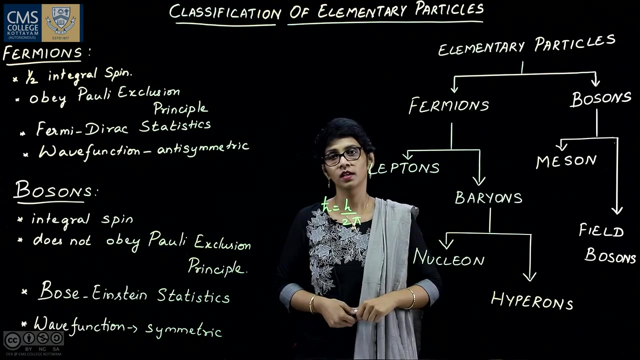 And its unit is h cross, where h cross is equal to h by 2 pi. Particles which have odd half integral spin are called fermions and those which have integral spin are called bosons. These fermions obey Pauli's exclusion principle. 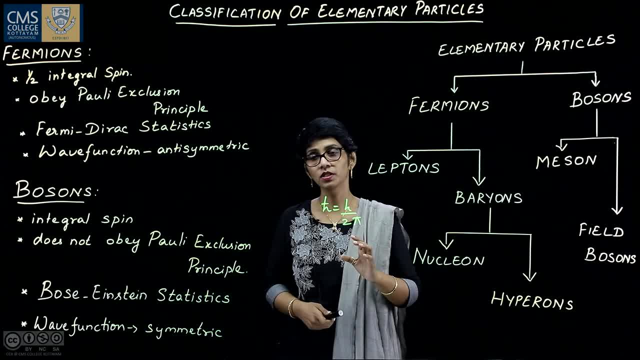 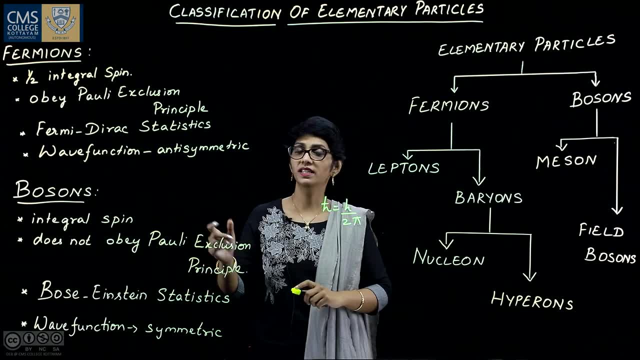 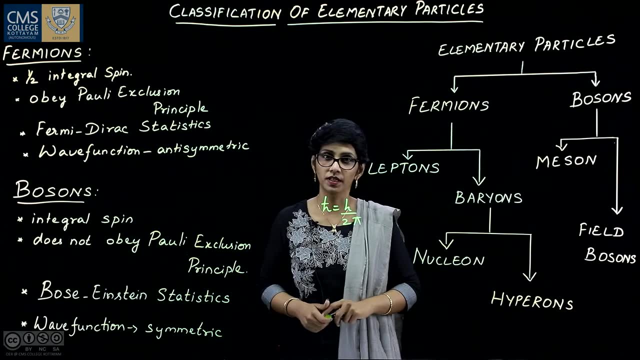 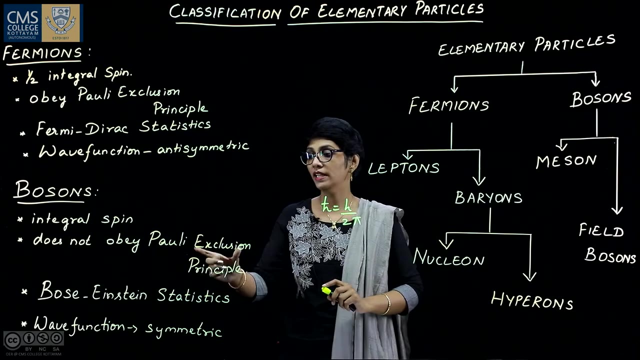 That means no two identical fermions can occupy the same quantum states. Also, these fermions obey Fermi Dirac statistics. The wave function which describes the fermions is anti-symmetric In the case of bosons. the bosons are not constrained by Pauli's exclusion principle. That means the number of bosons. 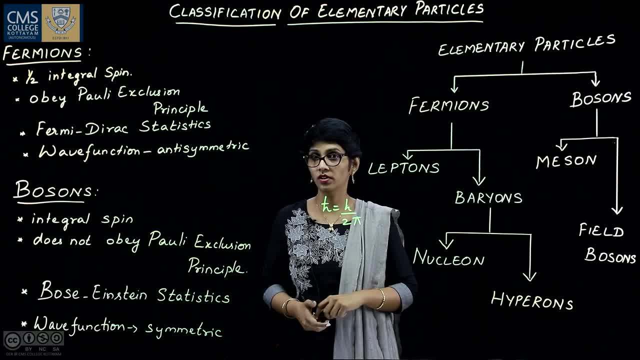 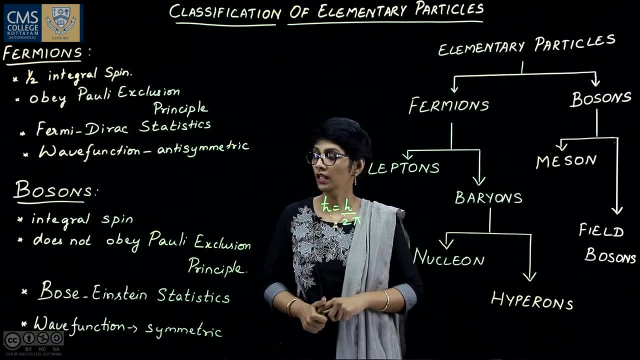 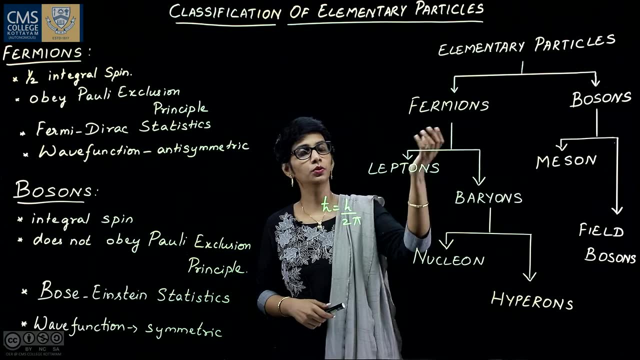 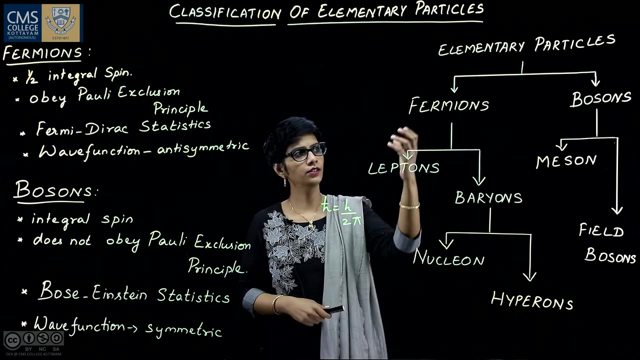 in any given quantum state is not restricted. These bosons obey Bose Einstein statistics. The wave function of bosons is symmetric. Fermions are usually associated with matter, while bosons are force carriers. These fermions are further classified into Leptons and Papill Credit cards. 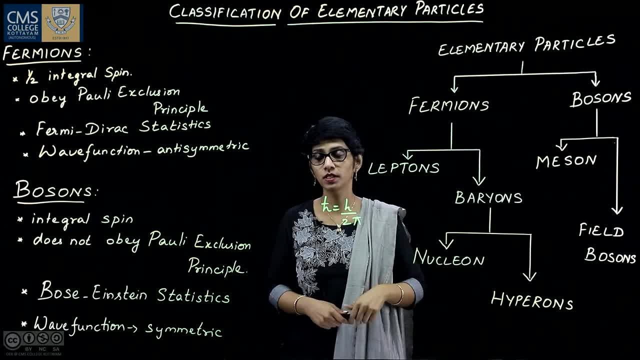 I guess this would be an interesting ci curls Потому Nobel 马比 特力诇学千回音 布出对 堕空反ème Sacrifice Track into leptons and baryons, based on the mass. 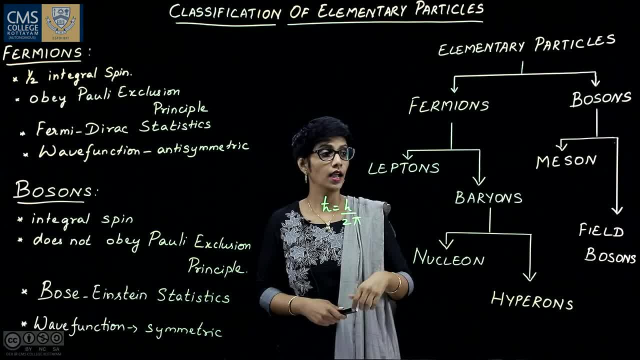 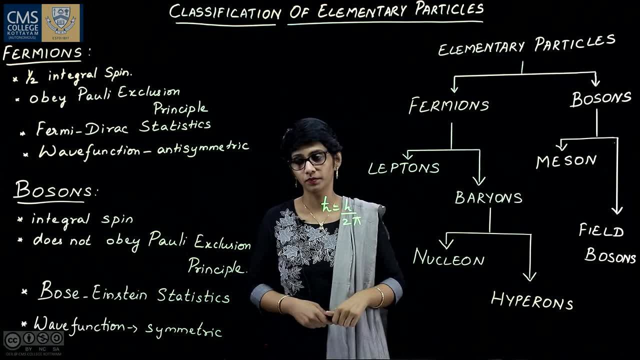 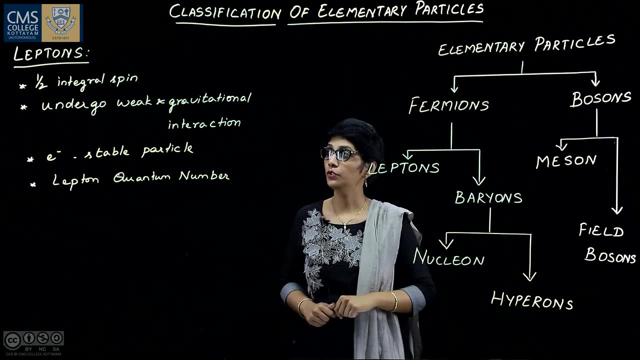 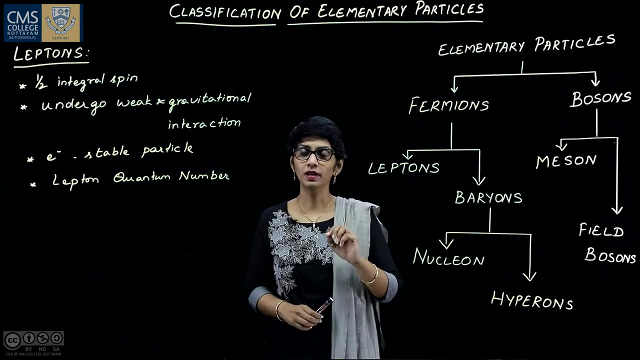 These leptons have mass lesser than meson and these baryons have mass heavier than mesons. Now let us see the leptons. Leptons belonging to fermions have half integral spin. These leptons undergo weak and gravitational interactions. But if the fundamental particles are charged particles, then they are affected by electromagnetic. 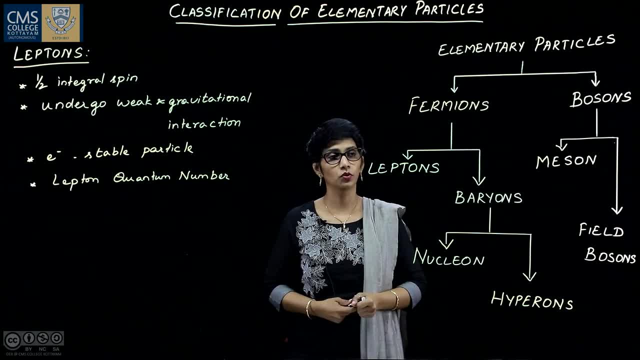 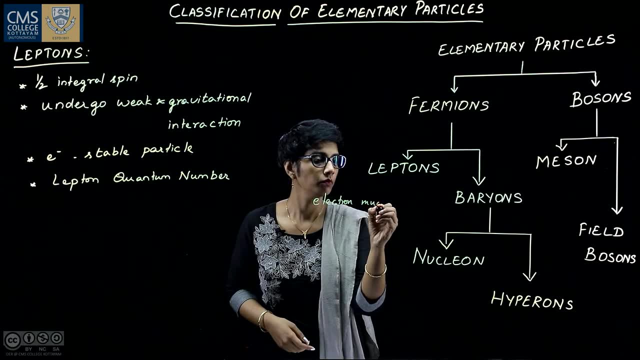 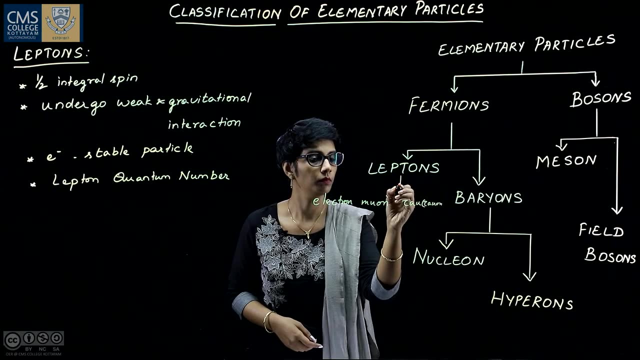 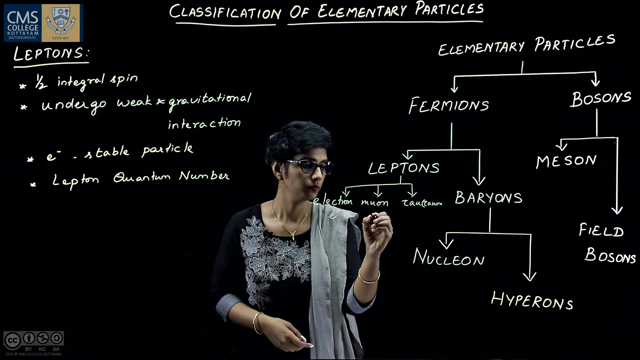 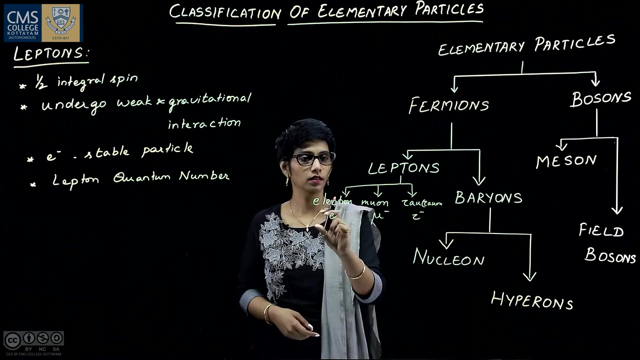 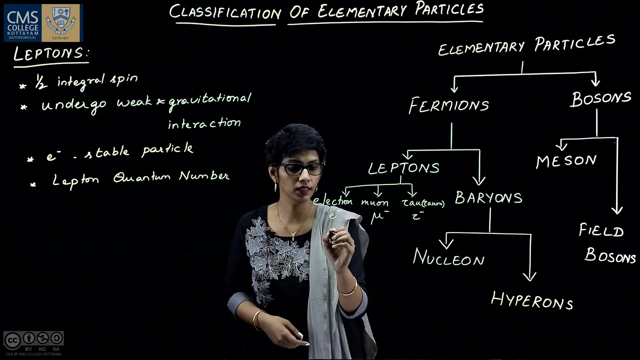 interactions too. The members of this lepton are electron muon and tau or tauon. They also have electron muon and tauon. Other have electrically neutral neutrinos, ie whether electron means electron neutrinos, is aone or is mue. 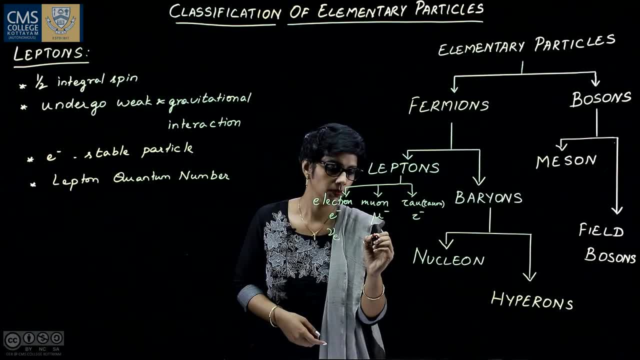 Vere are electron prophetic leptons. Electron Hue, Electron buyer For muon: the muon neutrino is nu mu, nu mu For tauon. the tauon untrot publications of neutrinos are 6 mu mu mu mu. So the Мих2V and illegot neutrinos are always neutrinos like this. 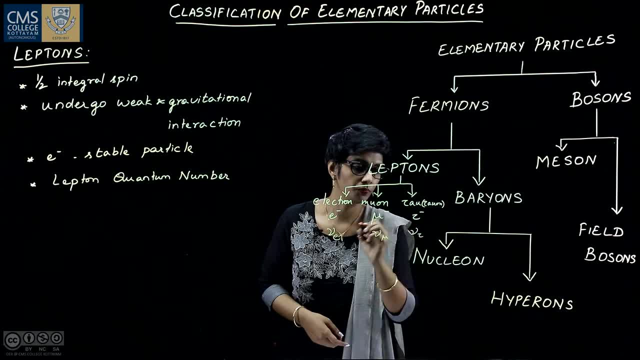 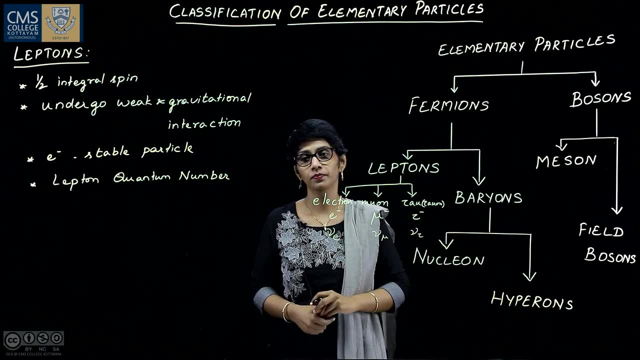 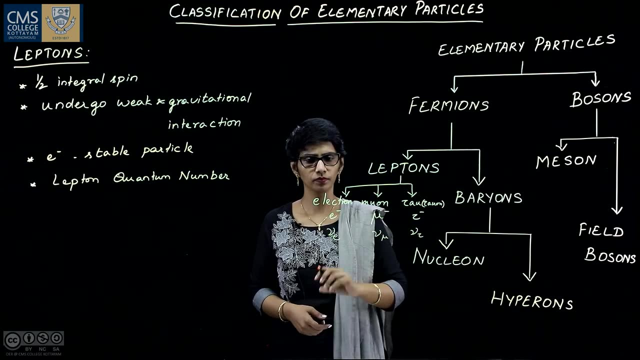 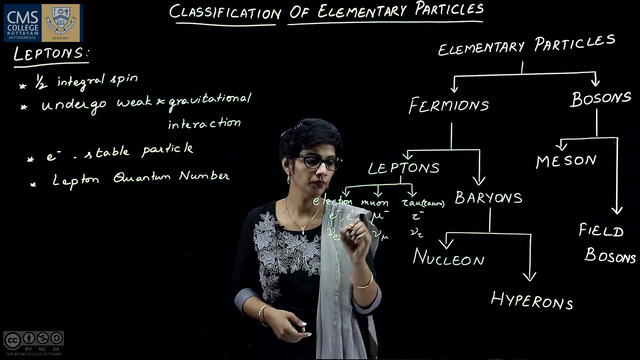 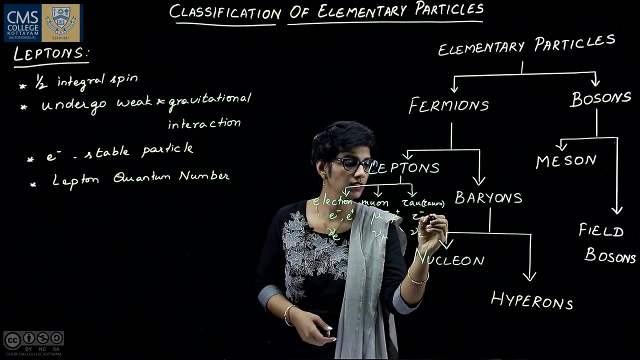 tau neutrino is mu tau. So there are 6 leptons. These 6 leptons have antiparticles. The antiparticles have all the properties of leptons except the charge. So electron is having antiparticle. positron and mu minus have the antiparticle. mu plus and tau minus have the antiparticle. 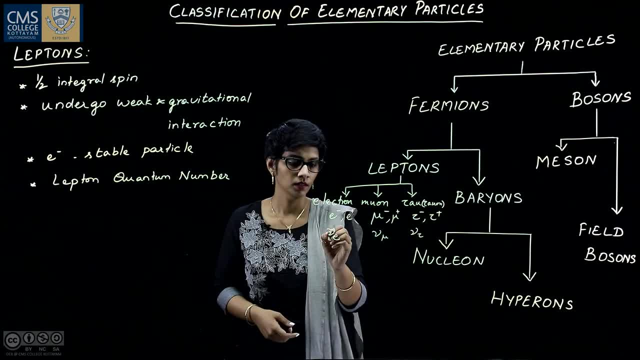 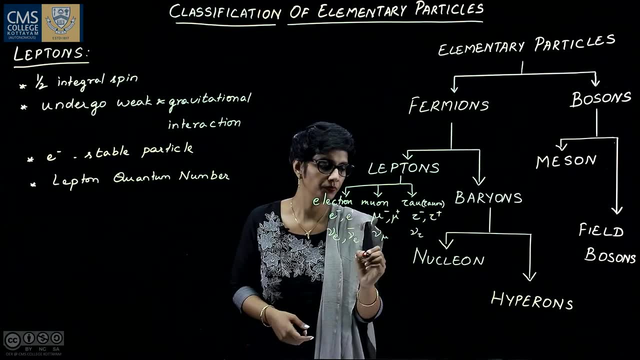 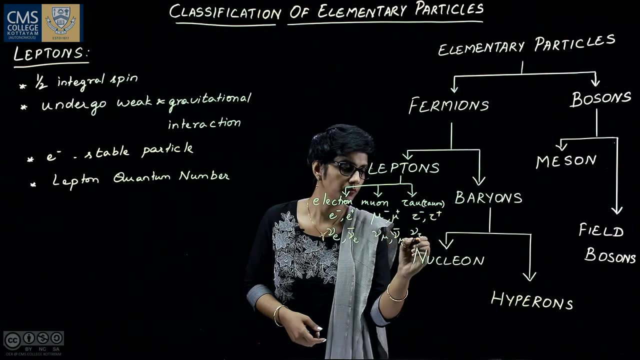 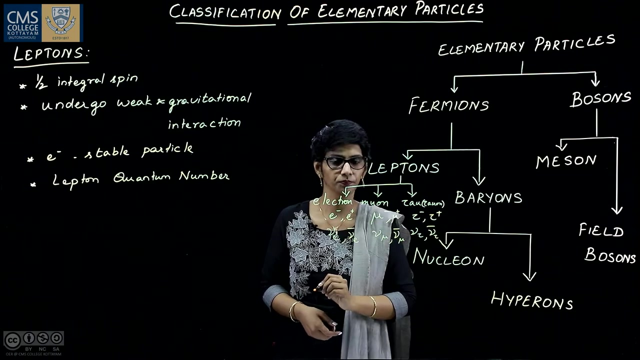 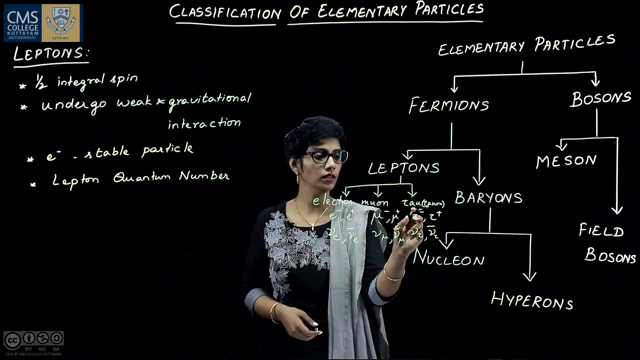 tau plus. Similarly, the neutrino. electron neutrino have antiparticle nu e bar and the mu 1 neutrino have the antiparticle nu mu bar and the tau 1. Tau neutrino have the antiparticle mu tau bar. These electron mu minus and tau minus have negative charge. 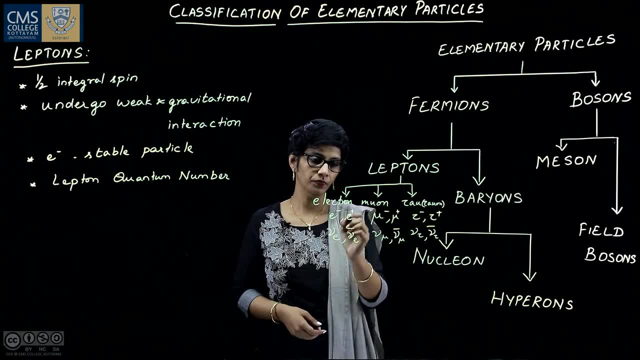 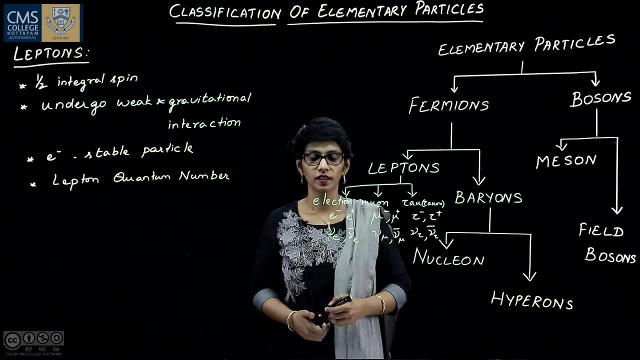 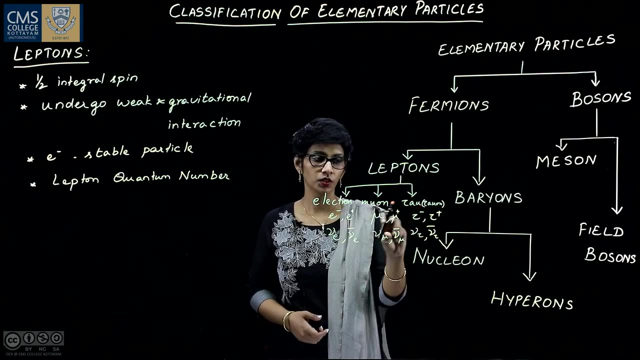 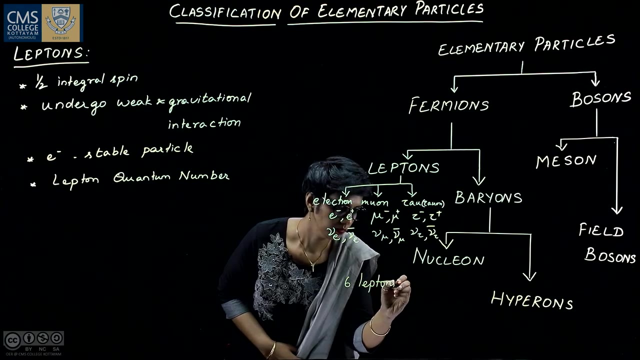 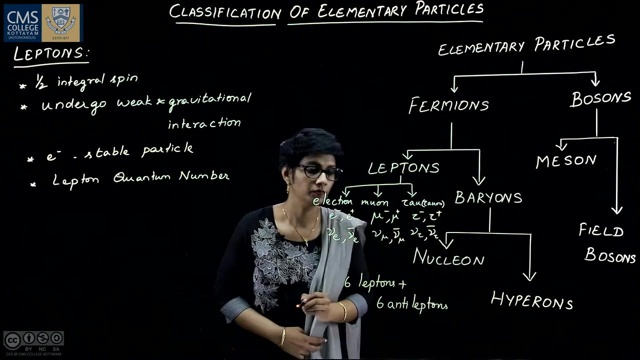 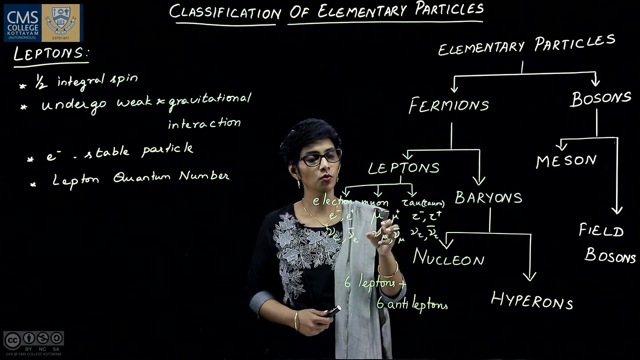 and these antiparticle, that is the positron, mu plus and tau plus have positive charge. So this neutrinos with the antineutrinos are electrically neutral particles. So there are 6 leptons and 6 antileptons Here. electron is the most stable particle. These tau and 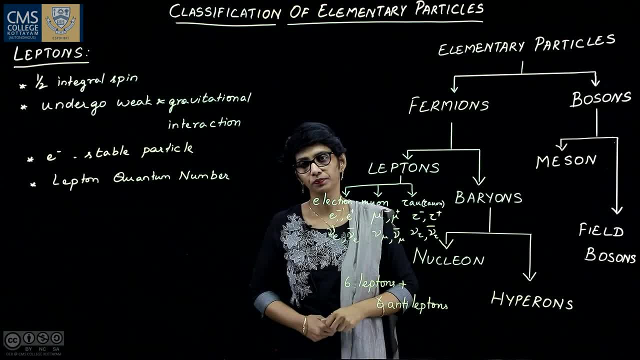 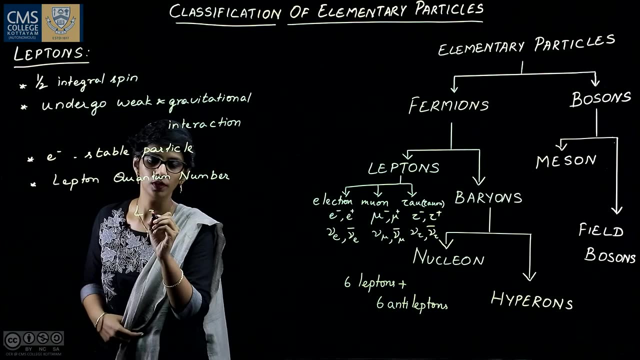 muon are electrically neutral particles, So these neutrinos with the antineutrinos are electron decay to electron. In particle physics lepton number is used to denote whether the particle is lepton or not. The leptons normally have lepton quantum number l equal. 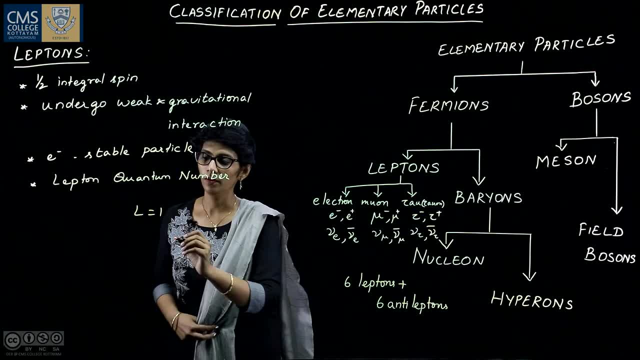 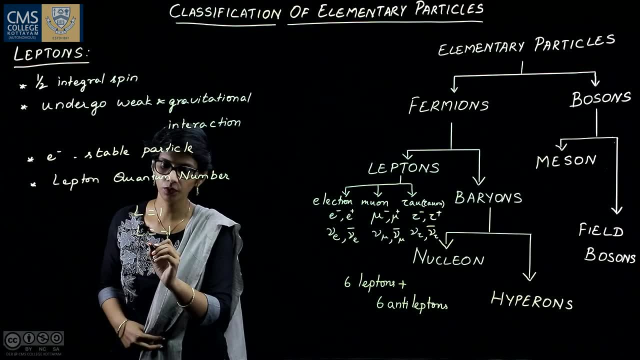 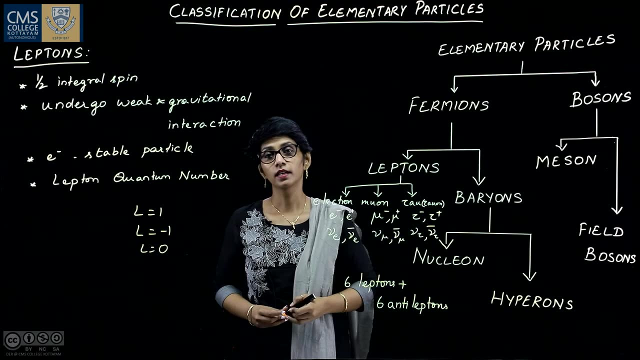 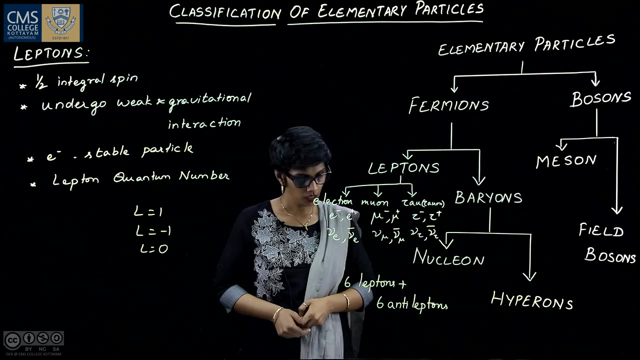 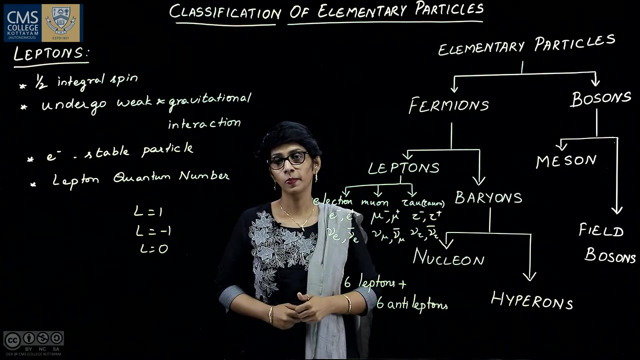 to 1.. For antilepton: l equal to minus 1.. For particles other than leptons: l equal to 0.. The lepton number is a conserved one in all particle reaction. Conservation of lepton number means a lepton of a certain generation can be destroyed or created Along with that. 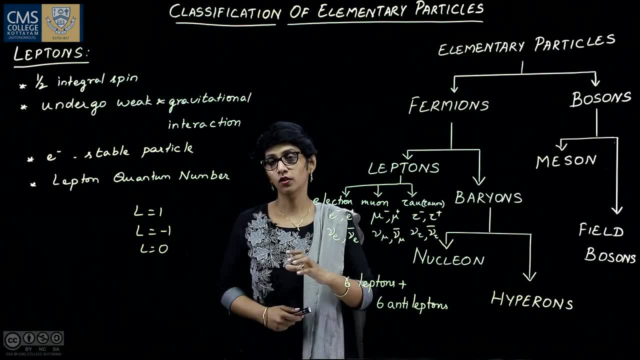 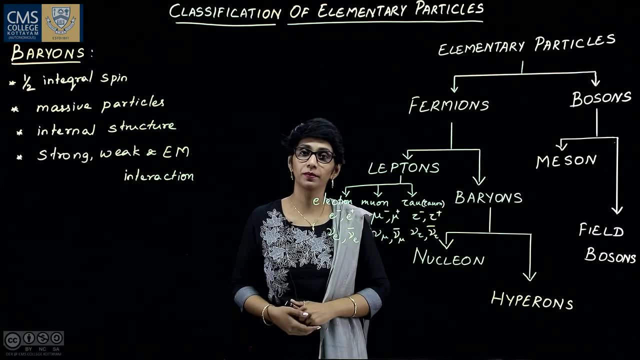 an antiparticle of the same generation should be created or destroyed. Baryons, belonging to the family of fermions, have high concentration of leptons, So they can be destroyed or half integral spin. They are massive particles and they are made up of quarks, and so they 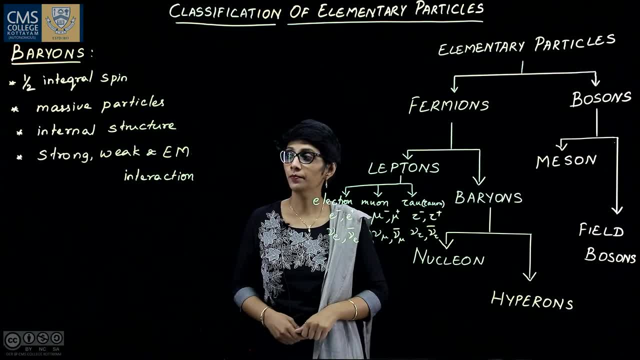 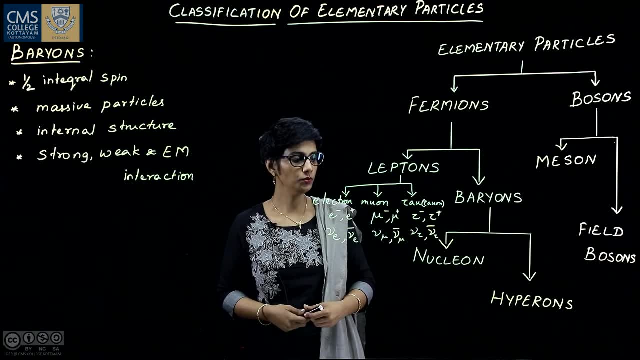 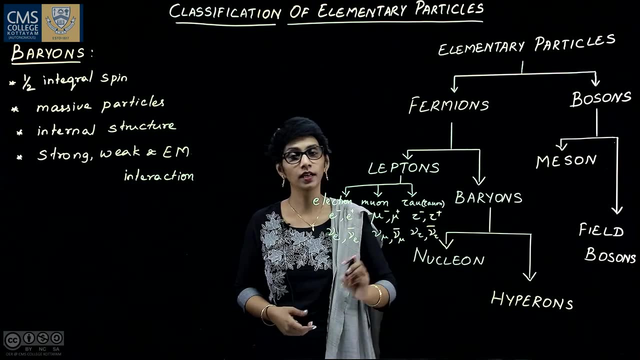 have internal structure. They are affected by strong, weak and electromagnetic interactions. These baryons are further classified into nucleons and hybrons. Hybrons are particles that are heavier than nucleons. These nucleons are classified into nucleons and hybrons. Hybrons are particles that are heavier than nucleons. These nucleons are. 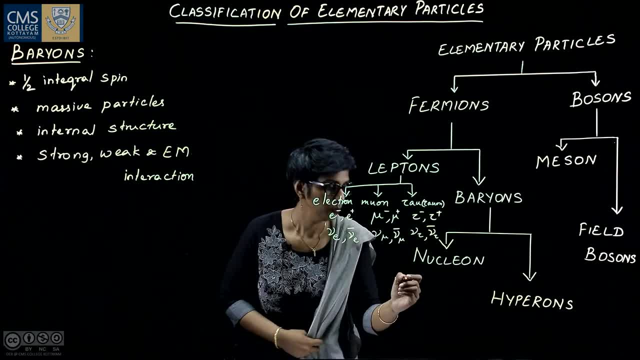 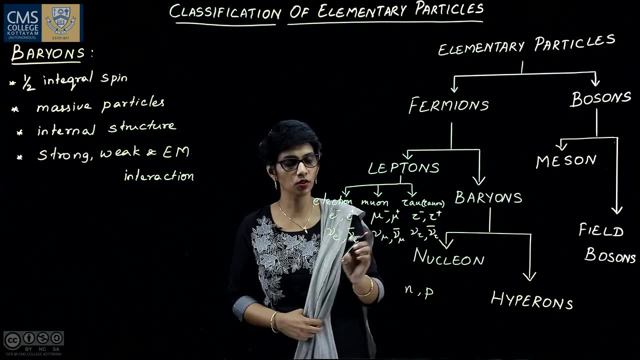 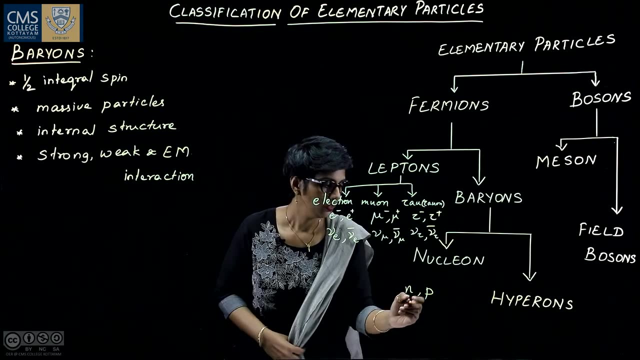 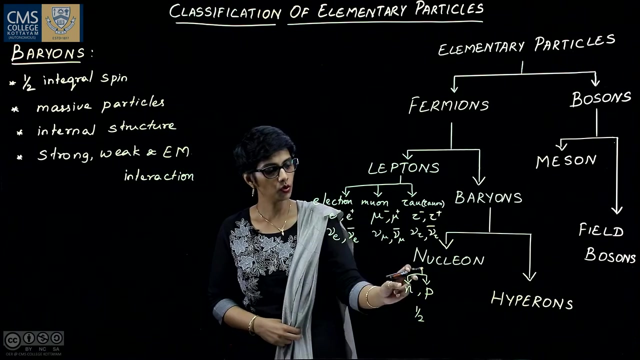 particles that are heavy than nucleons. Hybrons are particles that have neutrons and protons. They are present inside the nucleus of an atom. Protons are positively charged and neutrons are neutral. They have spin. half Scope is shown. It is possible that anything of the protein or the human molecule, as i showed you so far, 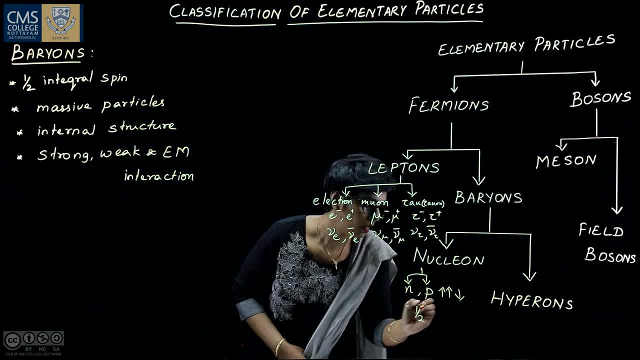 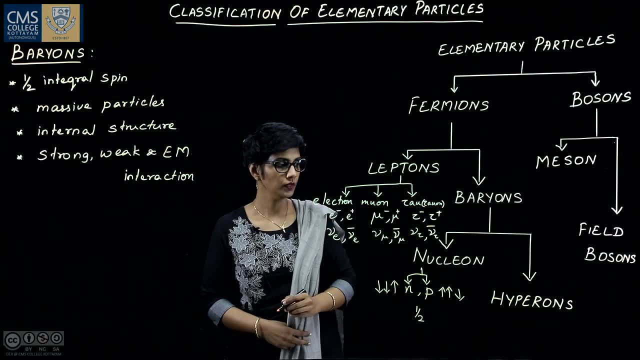 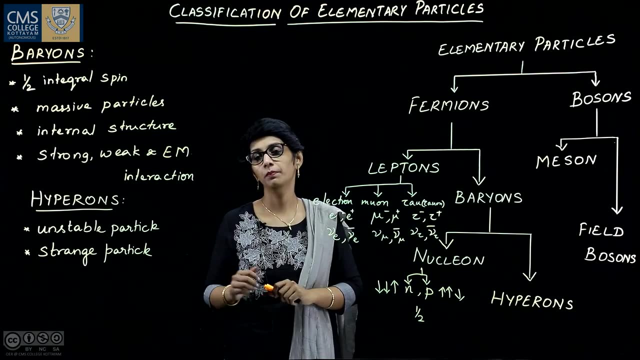 can have linear oppose those ofpace하며 2 up quark and 1 down quark. and neutron is made up of 2 down quark and 1 up quark. Now let us see hybrons. These hybrons are extremely unstable particle. 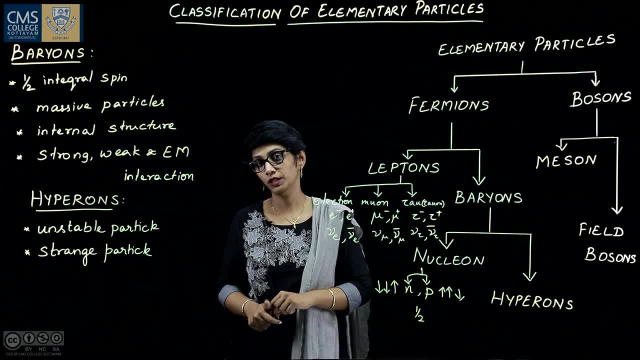 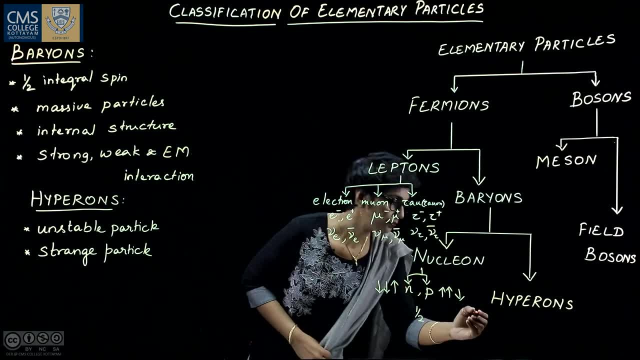 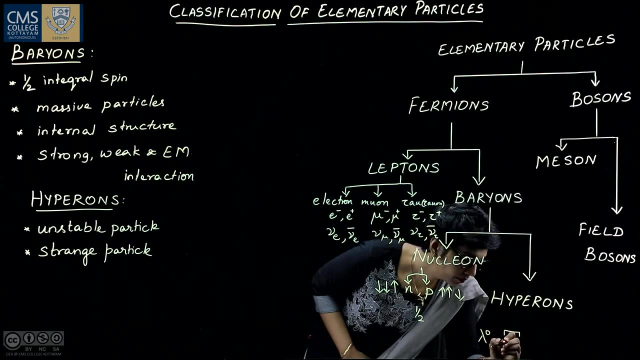 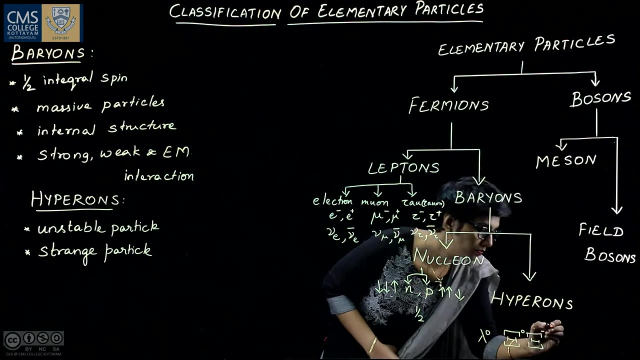 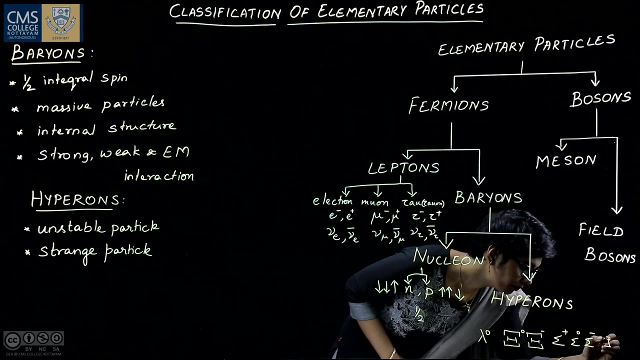 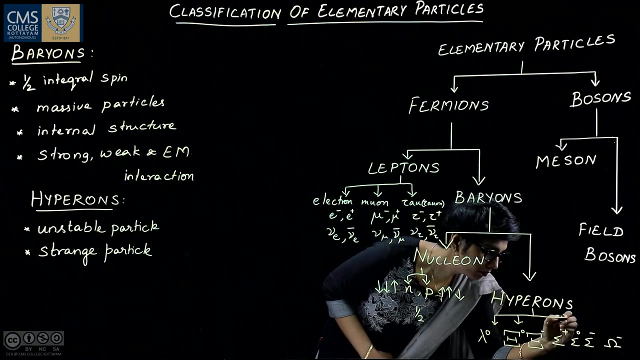 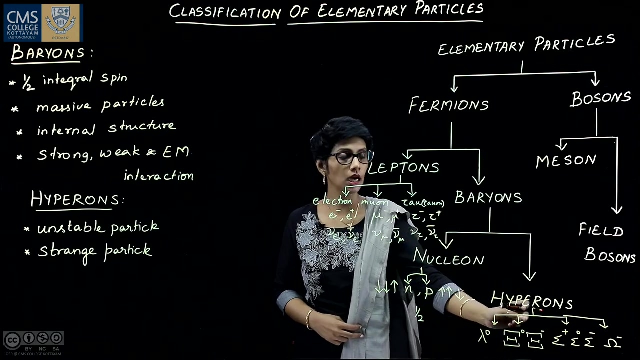 Their decay time is greater than the time of formation, and so they are called as strange particles. The members of this group are lambda naught, cascade hybron, sigma hybron and omega hybron. The superscript denotes the charge of the particle. Just like the leptons, these baryons. also have baryon number. For baryons, baryon number is b equal to 1.. For antibaryon, b equal to minus 1.. For particles other than b: b equal to minus 1.. For baryons: b equal. 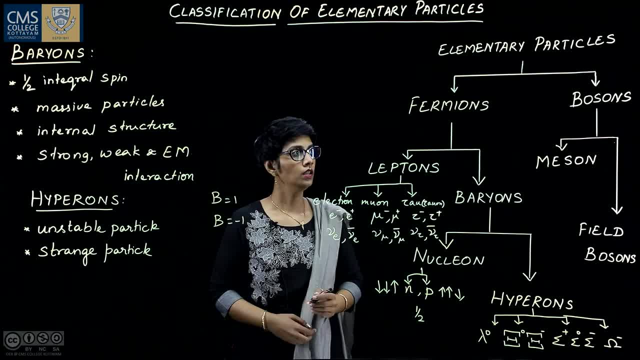 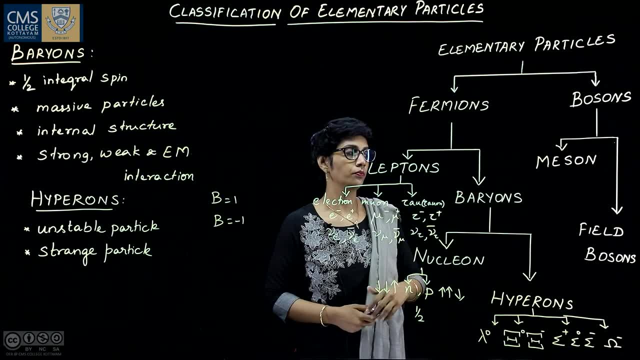 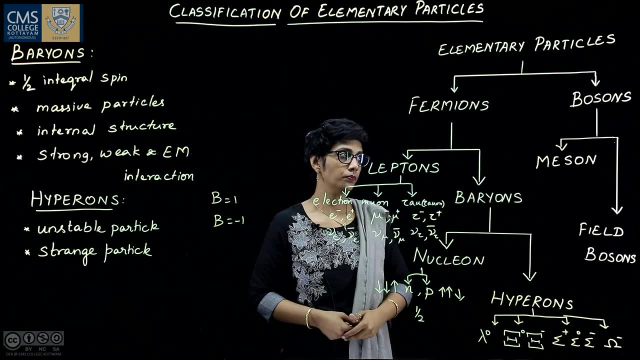 to minus 1.. For baryons: b equal to minus 1.. For particles other than b, b equal to 0.. Now let us move on to the next category, that is boson. Bosons are further classified into mesons and field bosons. Now let us see these two one by one. Mesons are particles. 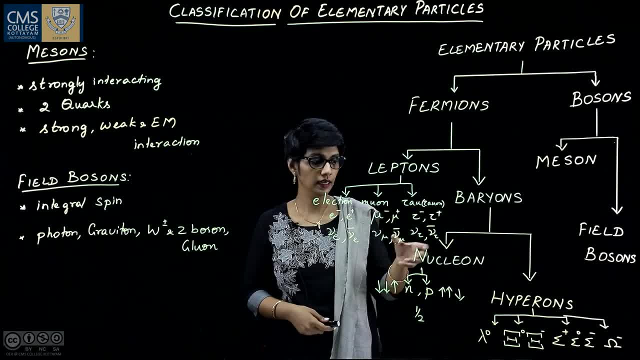 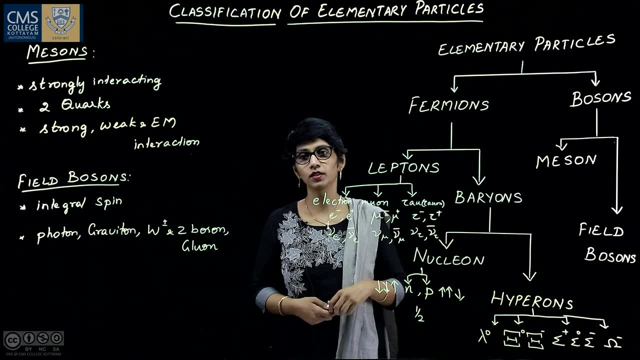 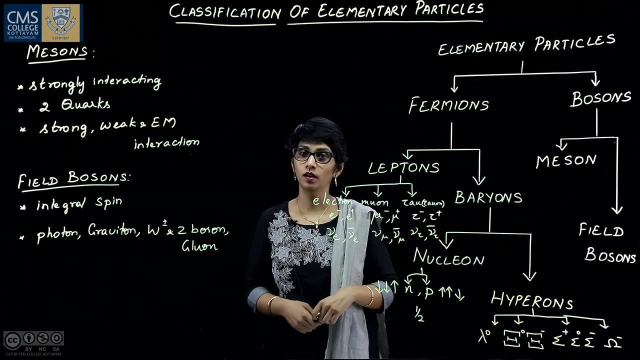 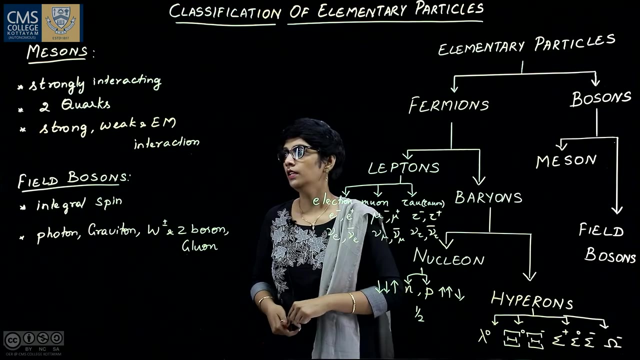 that are massive than leptons but less massive than nucleons. They mediate interaction between particles inside the nucleus. They are strongly interacting particle and they are made up of two quarks, One quark and its anti-quark, And so they have internal structure. These mesons are affected by strong, weak and electromagnetic. 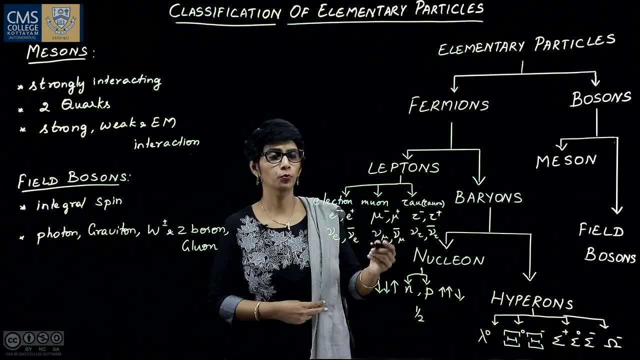 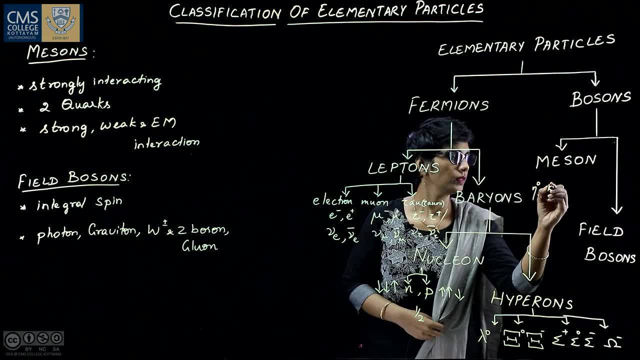 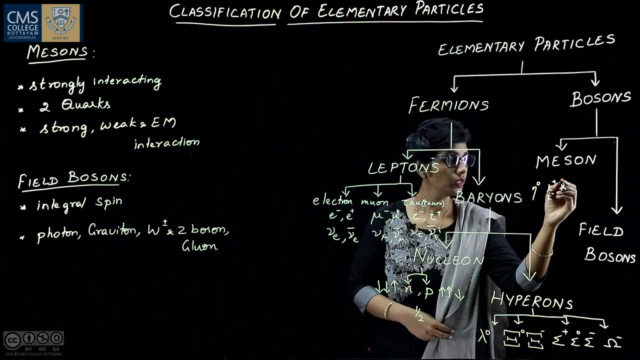 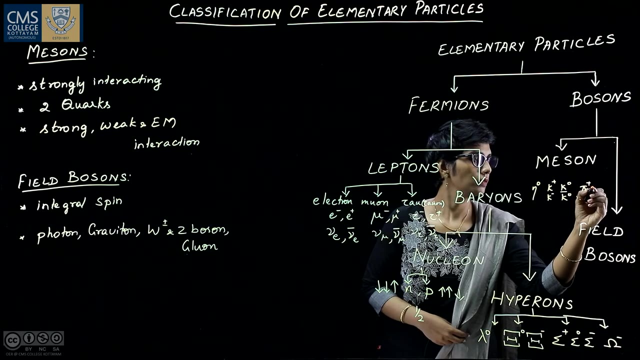 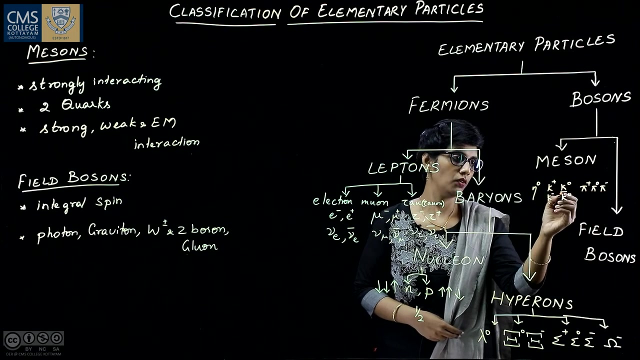 interaction. The members of this group meson are: Eta naught k plus k minus k zero, k zero bar, then pi plus, pi zero, pi minus. These are called as pions And these are called as kions: k plus k naught, k minus k naught.